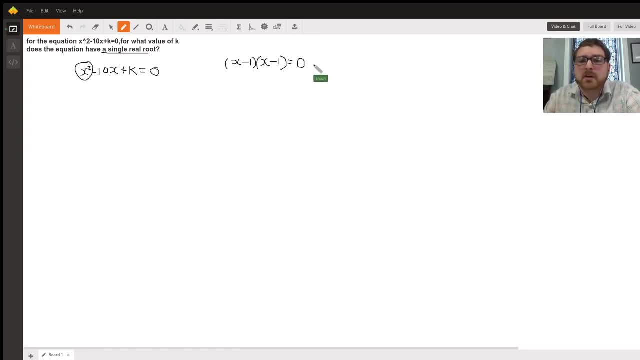 one. So that's an example of a case that's similar to this. So we need to find for our case here: x squared minus 10x plus k equals zero. What value can be set up such that x minus c times x minus c equals zero and is equal to x squared minus 10x plus k. That's. 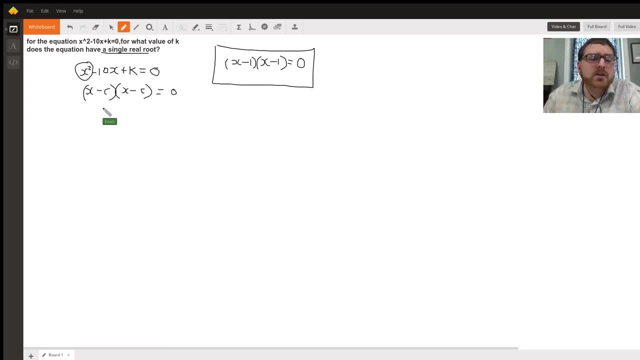 the basic setup we need. There's a couple of ways we can approach the problem from here. The way I would do it is to start in the middle, So I would start in the middle. I would start in the middle. The numbers have to add to this and they have to be the same. The only 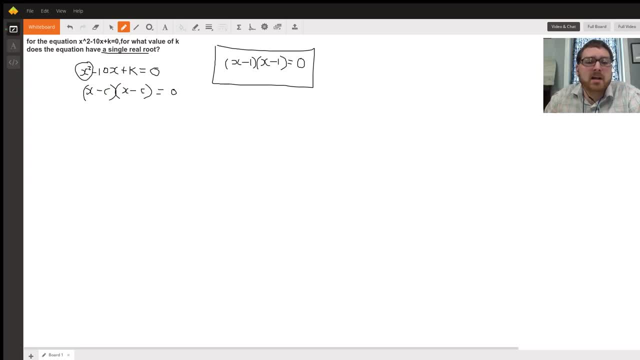 number that can add to negative: 10, when added to itself, is negative 5.. So then I would try: x minus 5 times x minus 5 equals zero. I can FOIL this: x times x is x squared. x times negative, 5 is negative, 5x Negative. 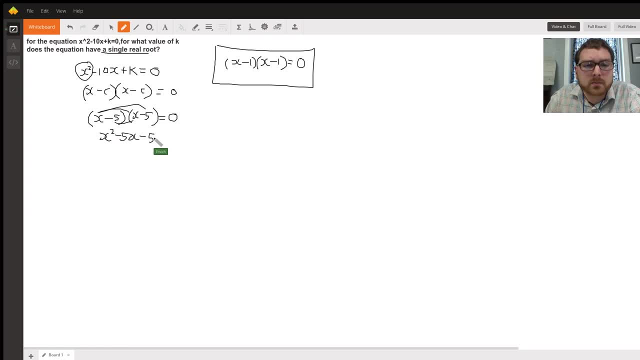 5 times x is also negative. 5x- That's what we were expecting. Negative times negative is positive, That's 25.. x squared minus 10x equals zero. Combining these, we get negative 10x. here The x squared. 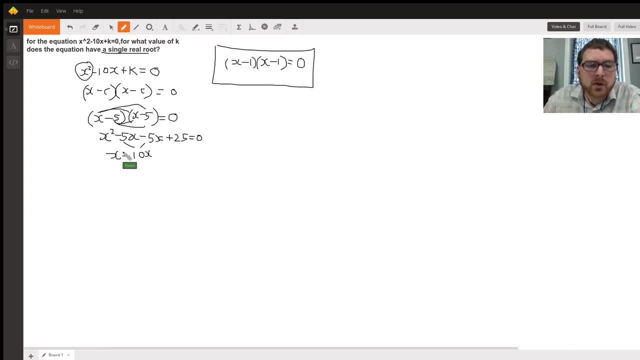 can come down: x squared minus 10x plus 25 equals zero. Now this is the same as our original problem, except instead of k we have 25.. And that brings us to our answer: k equals 25.. So a quick note on the key points here. First, we looked at our problem and we realized.